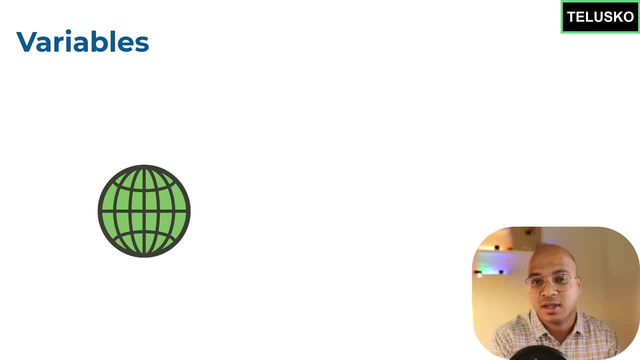 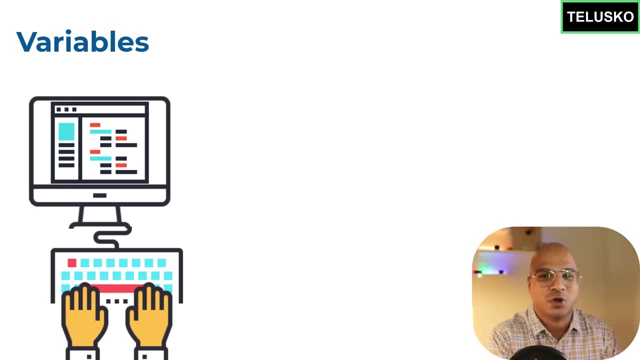 thing in IT or computers is information. So whatever we do, we do it for the information. You want to get the input, you want to show the output, you want to process data. It's all about data. right Now, the question arises where you will store data. Of course, with the help of programming. 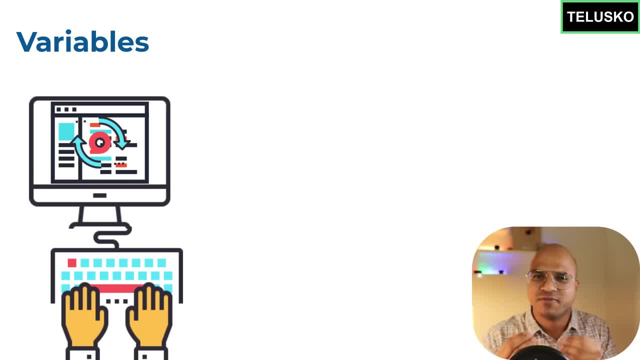 you can process data, But even for processing, first you have to store your data somewhere, and after processing you will store your data somewhere. So we need to store our data somewhere, and that somewhere is variables. The only tricky point is when you want to store your. 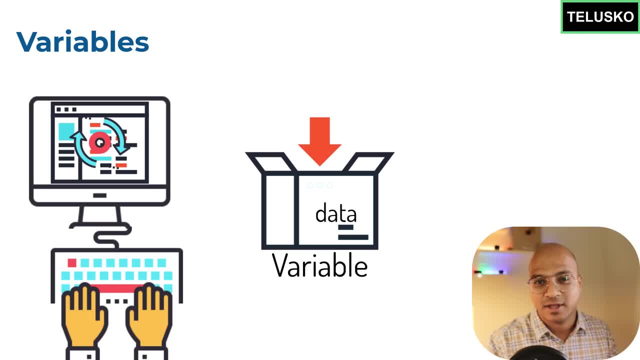 data for a temporary purpose, we will be using variables. If you want to store your data for a permanent use, we have different options for it. Currently, we are focusing on how do you store your data So we can do that with the help of variables. So, for example, let's say I have a data here. 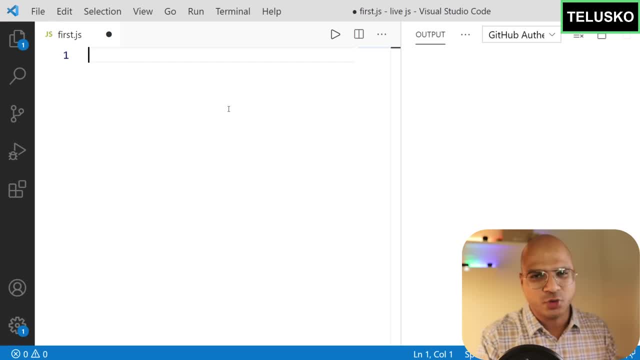 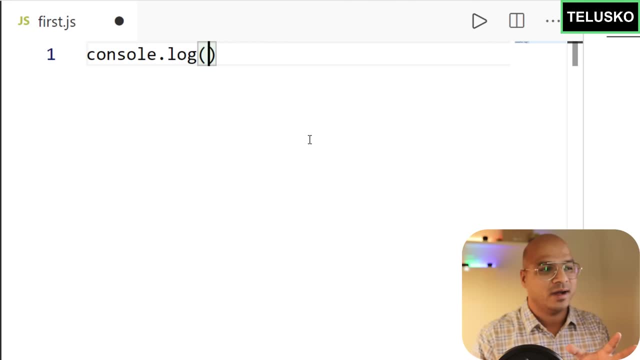 So let's say I want to perform some operations before doing that. So we'll add two numbers here first. So I also want to print them. So what I will do is I will say consolelog, The same thing we've done for hello world Here what we'll do is we'll say 2 plus 2.. 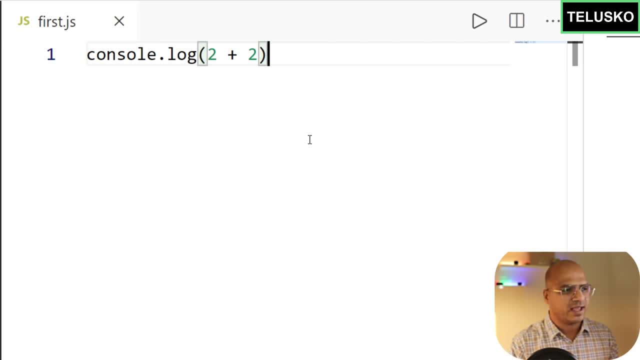 Now, of course, if you run this code, you will get the output right, So let's save this file as well. So we are doing the same file which we started, which is firstjs, which is available on desktop. Okay, so let me just run this. Of course, you have two options of running this. We can write: 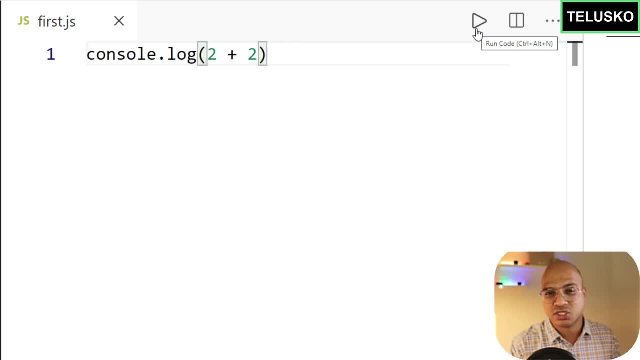 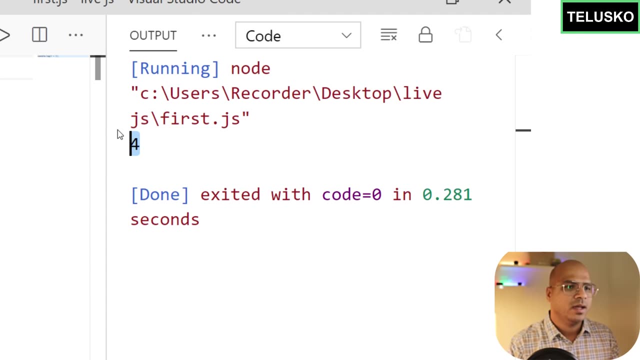 our node command or we have installed this extension called coderunner. Let's use that. So when you click on run, you can see we got the output as 4.. Okay, this looks cool, right, But then I want to store this data somewhere so that I can. 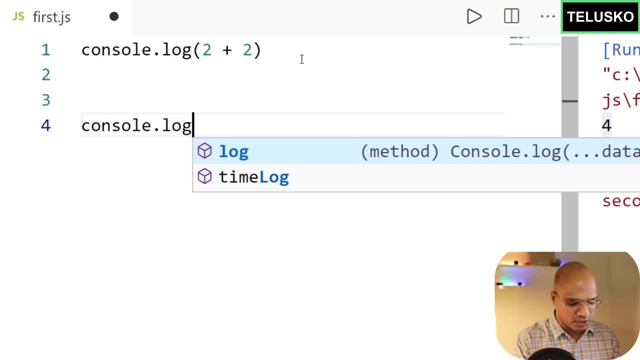 use it. Example where I want to use it Again. I will do a calculation here and here I want to add two numbers. One is a new value, Of course. let's say I want to add three, But I want to add this 3 with the previous operation. Maybe you have a choice. Let's say the previous. 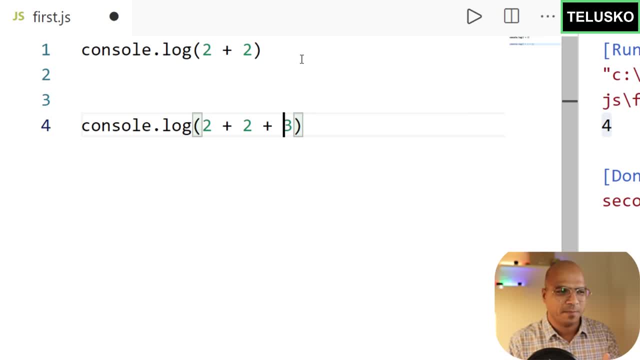 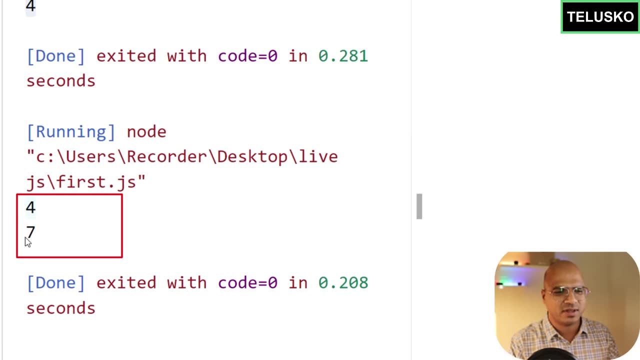 operation is 2 plus 2, and then you will say 3.. But don't you think you are doing the same thing again? Example: when you run this code, of course you will get 4, you will get 7.. 4 because of the first operation, 7 because of the second operation, But don't you think? 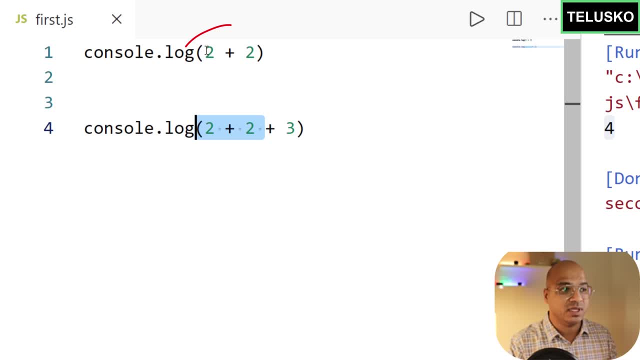 we are doing it again. So, basically, if this takes some time, even this will take some time. So what if you do this addition? Store it somewhere. So let's do that. What I will do here is before consolelog. I want to achieve this operation. I also want to store it somewhere. Now, where to store it? 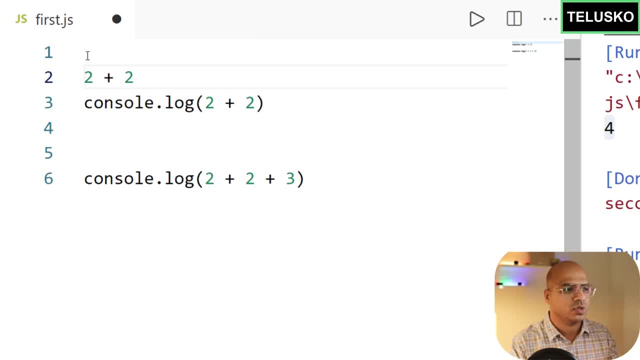 So we have a concept of variables, and variables has a name. So let's use a variable name. I will store this number in num. So let's say num equal to 2 plus 2.. So whatever you add here, which is 2 plus 2, will be stored on this variable or inside this variable. 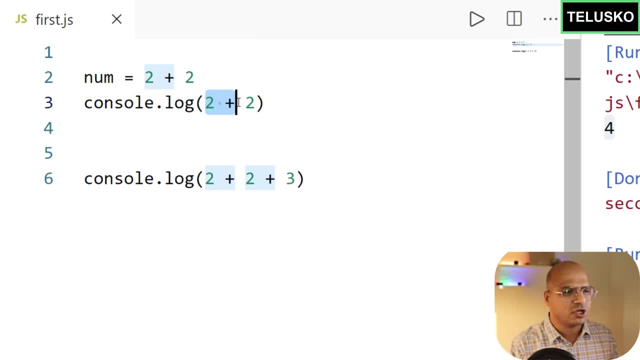 So this looks cool, right, And then I can just use: instead of printing 2 plus 2, I can print num here. So imagine this num as a box And inside that box you have a value now which is 4.. So this is an. 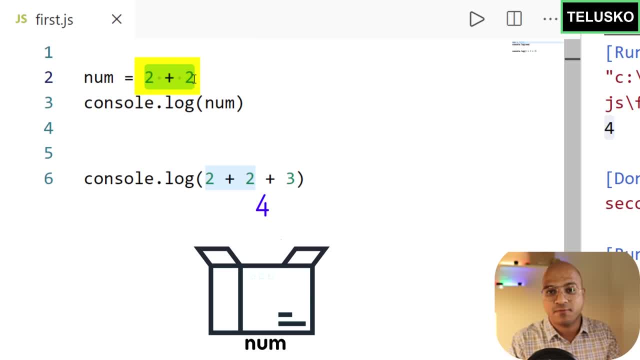 expression which will evaluate, and the value, which is 4, will be stored inside num, And then when you print num, it will print the value of that box. So box is num and what you get out is the value which is 4.. Okay, so now we can use the same 4 here, But before 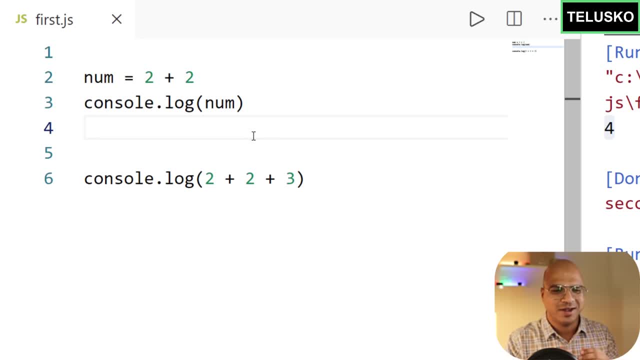 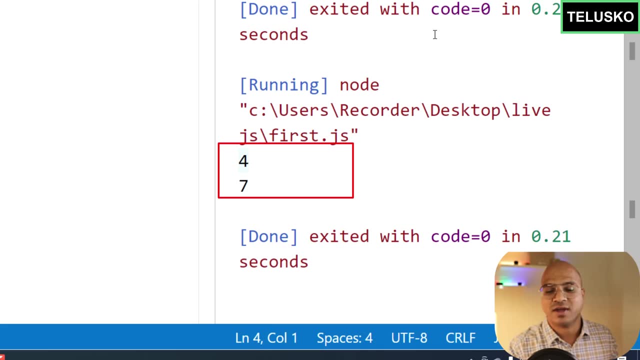 that. let me just run this To change. if that, we can also use the same value Here. let me check if everything is running. so whenever you do small changes, make sure you run it to check what is happening. so let's run this code. okay, at least we have not got the error. we got the same output. 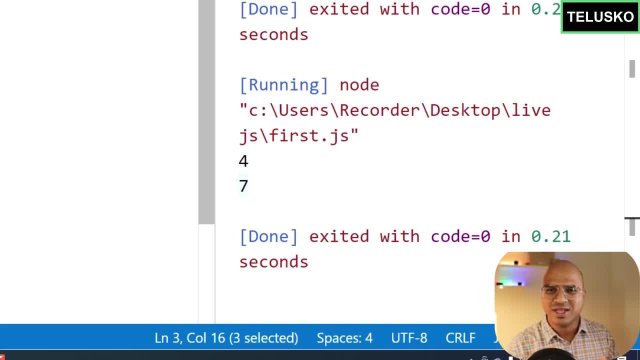 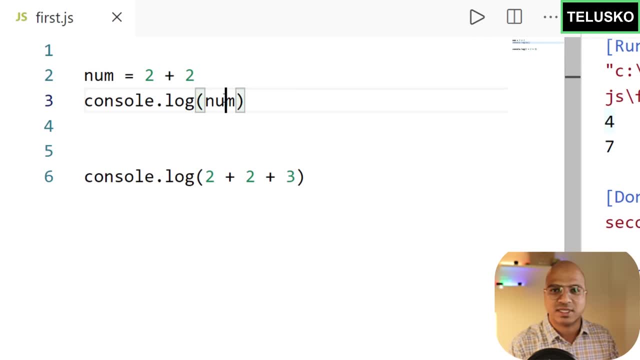 because we have not changed the operation yet. the only change is this time you are fetching the value from a variable, so the first for which you got here is coming from this num. okay, now i can actually reuse and that's the power, right? so once you have a data in the variable, you can use the same data. 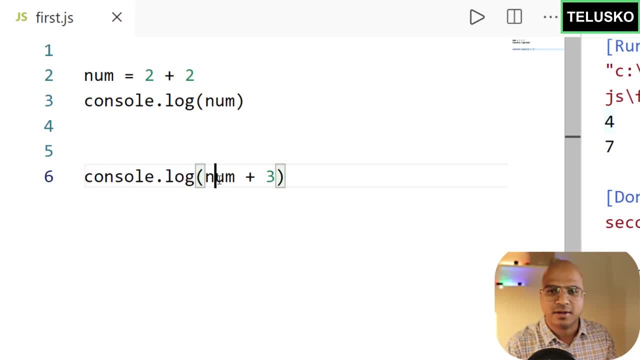 multiple times. we are doing it here. we are doing it here and you can use it again, not just for printing the value. you can also use it for addition, which we are doing here. you can do all the operations. the data will be there. okay, how long that your data will be there, is it the right? 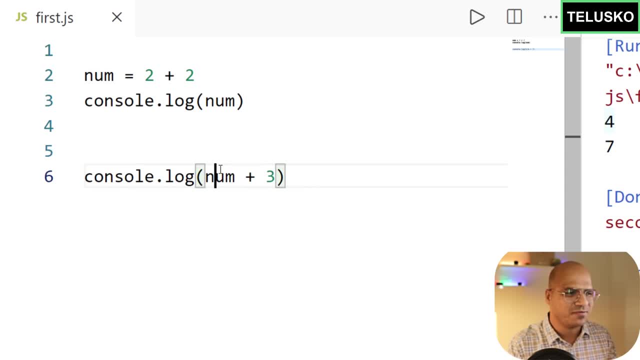 way of creating a variable. i will talk about that as well, but as of now it's running right. see, the most important thing is when you learn thing for the first time. so first let's understand what it is, and then we'll see how we can use it, and then we'll understand what is. 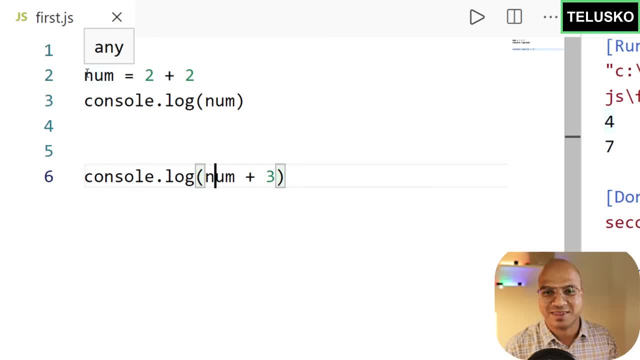 happening behind the scene. this is not a time to understand what is happening behind the scene, right? so let's go with the flow. we have a variable. imagine a box. you have a value, you're printing it here and you're adding it here, but is it the right way of creating a variable? see, if you want to. 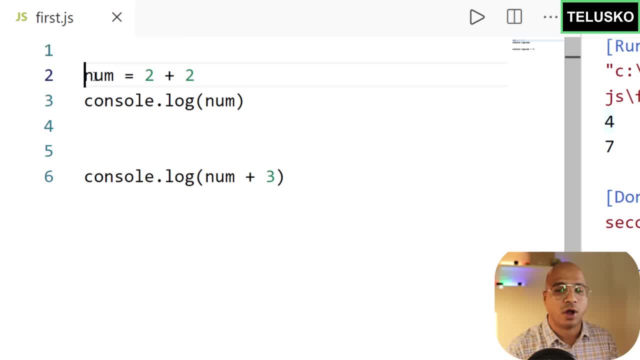 create a variable. in javascript you have an option of just by saying a variable name. you can use it by chance if you're coming from another language, let's say c, c++, java or any language which needs you to declare variables. that's right. in some languages we have to declare them first. here we're not doing that. we are simply saying: 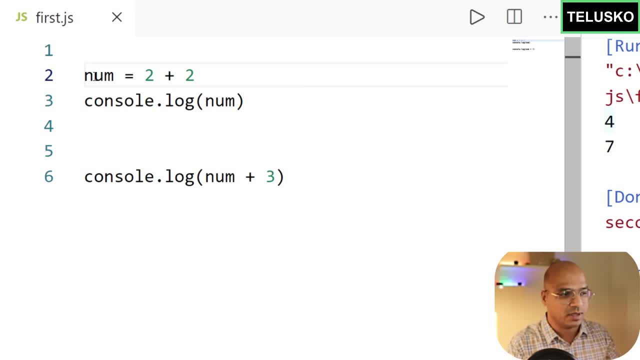 num. but this is not the right way of defining a variable. it is allowed here, but then with every new version you get new features right. so this was an old feature. so if you want to get a variable, say let, so it's a let num equal to whatever value you want to assign. so basically, this let is a. 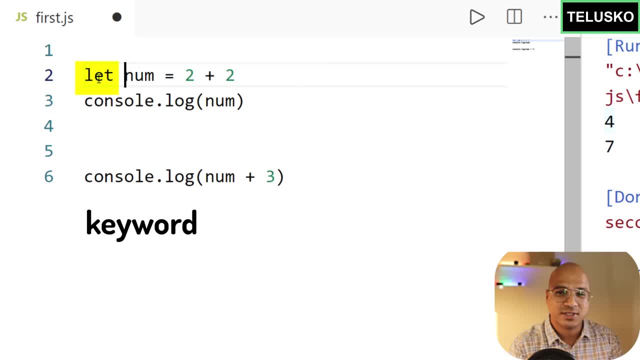 keyword using which you can create a variable. there's other option as well, but we'll see that as well. so in this case, here we come back and we start with assign name first, a variable right and two items into the list. so i will just name it isn't wanted, so that when i create a complete 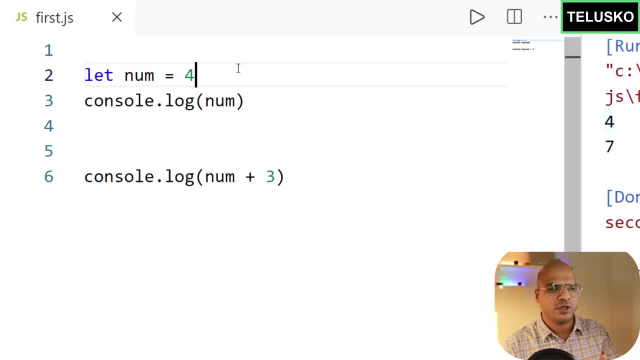 variable name. i can calculate it only, and then I can create the variable name first. okay, i will just say num, but this is pleasant for a lot of things, so you need really think i can do that. so right, once you've created, which means let us say it's like magic wizard, it's something. 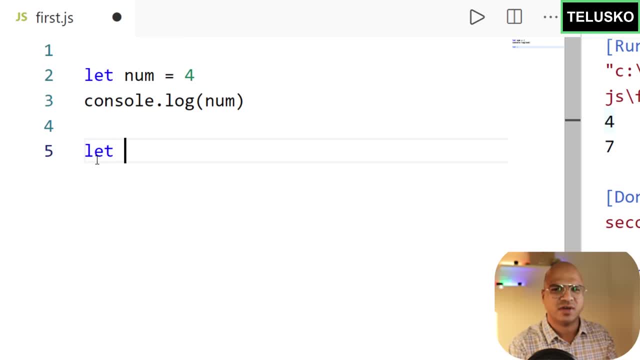 really cool. i will come over to web explorer here. let me actually create one. let me just add some more parameters in my browser express and put a name to that c so i can directly us if you have value named, value assignment, and you don't have to always create a operation or create an expression. 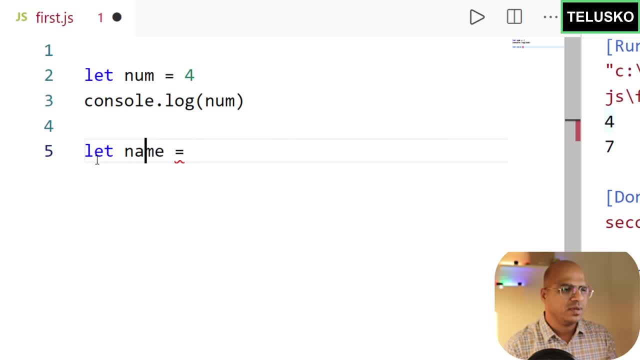 here i will say: name is equal to okay. now the problem is: name is a inbuilt keyword, so let's use something else. let's say, let's say user, and this is important. make sure that you always name your variable properly. maybe you can also use a, b, c for a smaller code. it works. but then the moment. 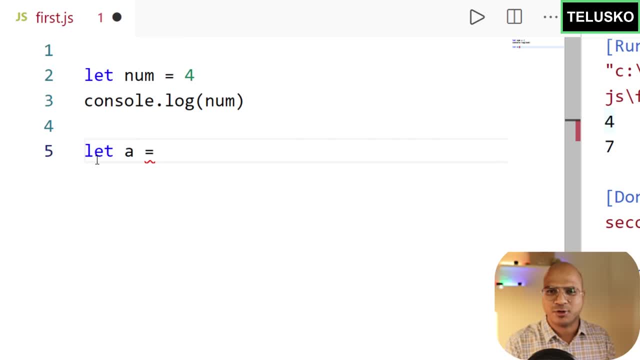 you have lengthy code, it will be difficult to guess what you're trying to do, so don't use a, b, c, something like that. always use proper names. maybe you can also say username, right? so let's say this username. i want to store my name, so the way you can do that is by saying you can mention a name. 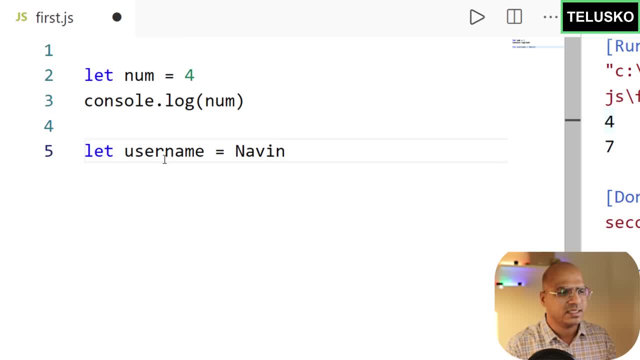 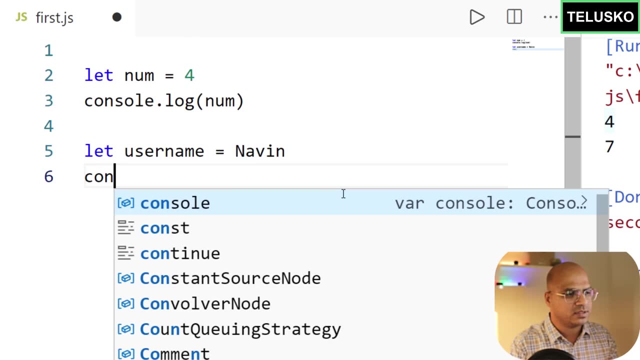 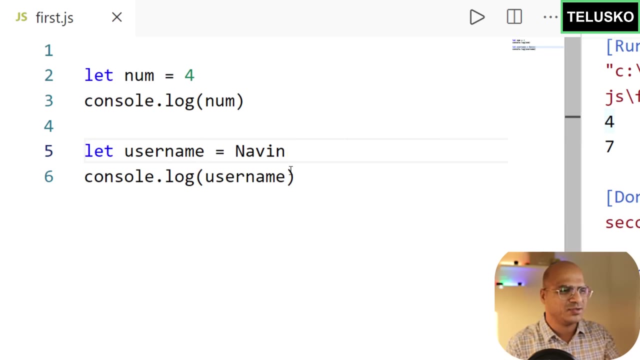 here. so my name is navin. so i will simply say: let username is equal to navin and let's try to print this. i will come back here, i will say console dot log and i will say username. what do you think? will it work? it should, right. i mean, everything is working as of now, so let's run this. 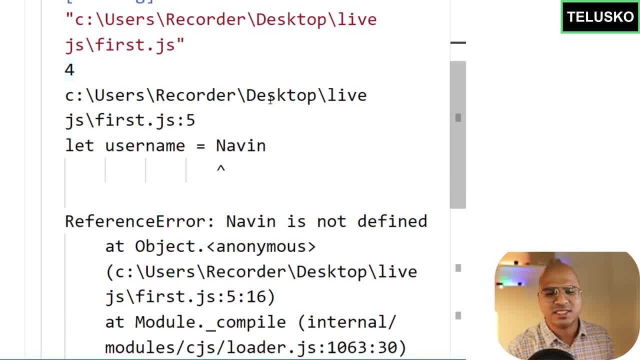 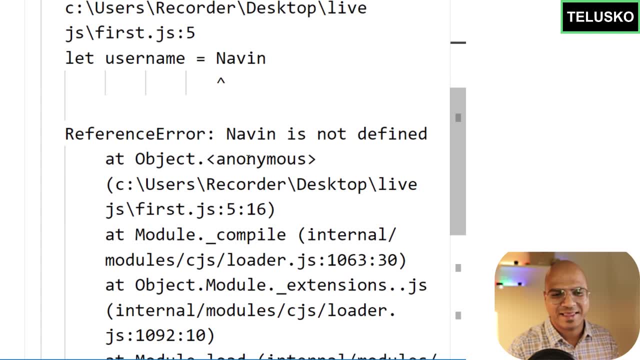 code and let's see what happens. and the moment you run this code, oh, this is your first error. congratulations, this is something. if you're doing programming for the first time, this is something you'll be doing in your lifetime, right? so as a programmer, you write code and you face errors. okay, uh, i don't. 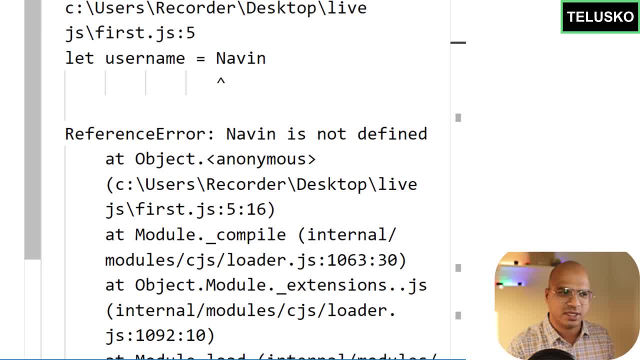 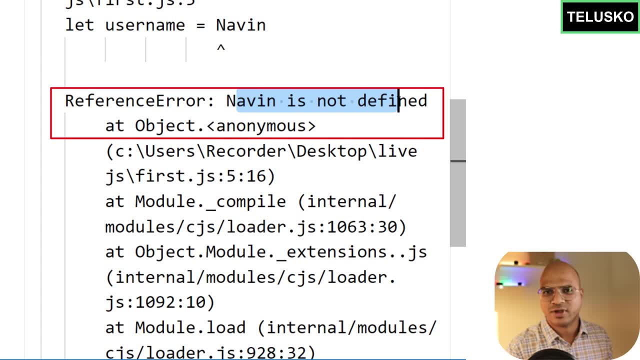 want to scare you here, but we have a variable username and then we are trying to assign a name and we got an error. see what this error says. it says navin is not defined. that's where i am defined here. uh see, the problem is, if remember, we have talked about this- whenever you write a code that 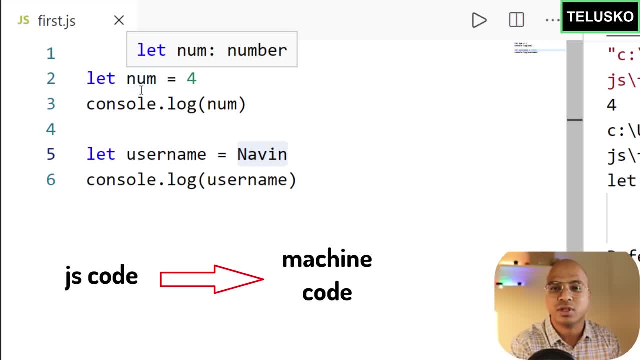 code has to be converted into a machine code, because the computer understand only one language, which is machine language. so your engine, which we are talking about, will try to convert this code into machine code, right? so it will start in this way. so it will say: okay, let, let is what it's a keyword, right? so it knows what that let means num, okay. 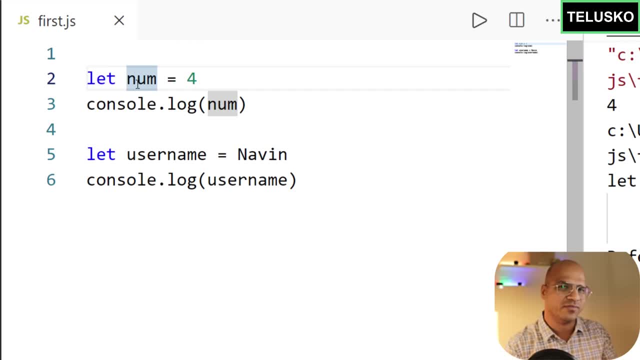 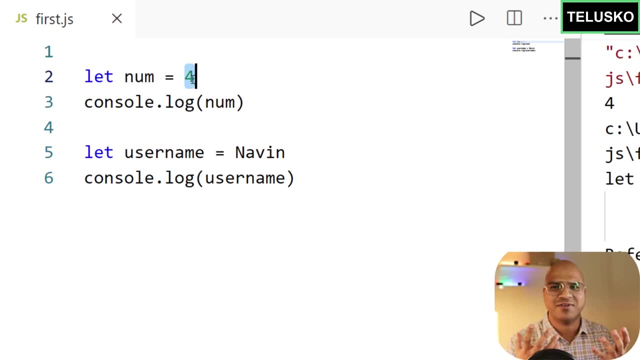 it knows whenever you have a let keyword. after that, when you have num, it's a variable name. so javascript knows about these things. equal to is in inbuilt code is a number, right? so of course we have finite numbers. uh, then we have console. again this is a variable name, so we have a variable name. 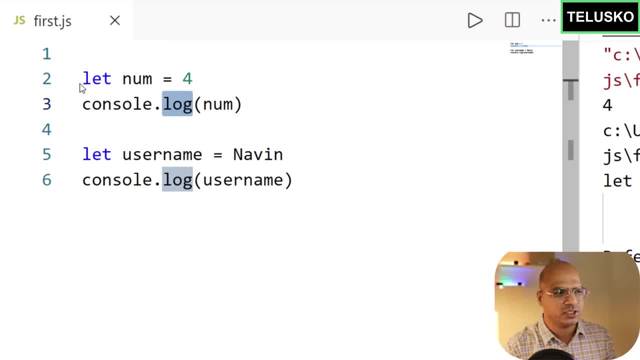 in build. log is in build, so everything which you can see on the screen, so even this, let is known to the javascript. this username is a variable name, so it will accept it. the moment you say, navin, it got confused, it is confused. is it a variable name? is it something which which a user has defined? 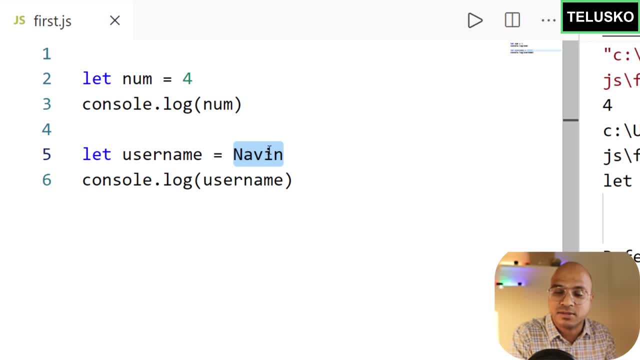 this. so there are so many things which is defined by the javascript and there are so many things which you can define. example: num is my creation, username is my creation. what about console log inside your javascript engine? the moment you assign navin? it got confused. is it a variable name? 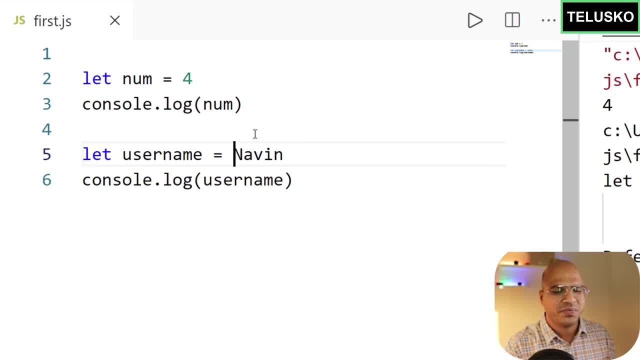 so we have to say, hey, don't treat this as a variable name. treat is as a string, something which i want to assign. example four is well defined. right, we have a finite number, but strings it can be anything. right, it can be a lengthy name. example: my full name. 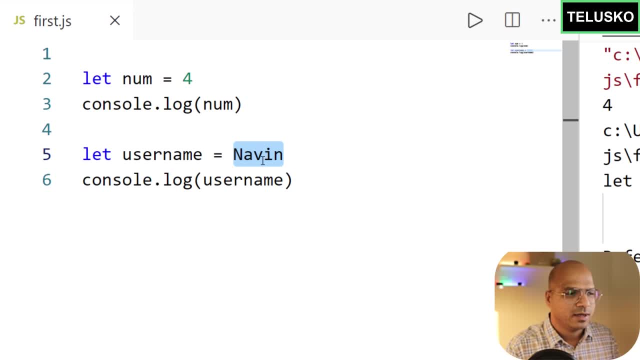 okay, i will not repeat that, but it can be anything. so when you want to assign a string, always use double quotes. so text string it should be inside a double quote. now you have an option. you can use double quote or you can use single quote. okay, it's your choice. javascript says you can use both. 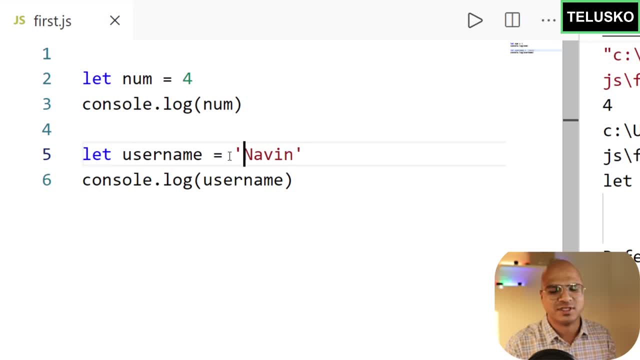 and that's why javascript is a flexible language in that case. but yeah, if you are using a double quote at the start, don't use single quote at the end. okay, so either use single quote or double quote on both the side. and now it should run, because i'm expecting it should be giving an. 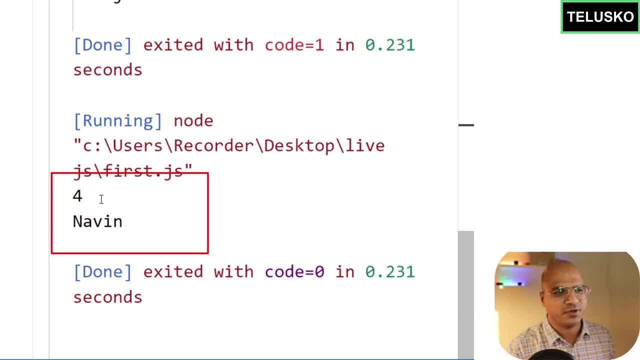 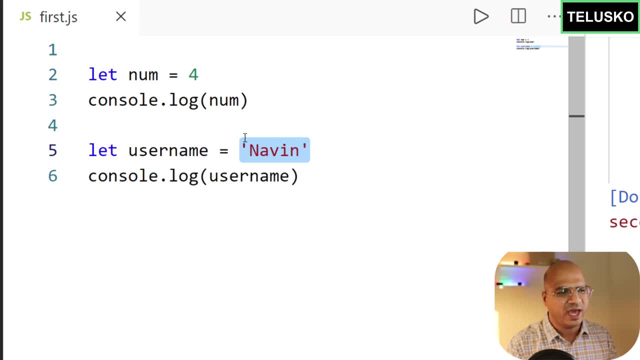 output. now, if i scroll down, you can see it worked. we got four and we got navin. so that's how you store a string or a text: use single quote or double quote. now why we have two options. example: let's say i want to store navin's phone or navin's account, so in that case i 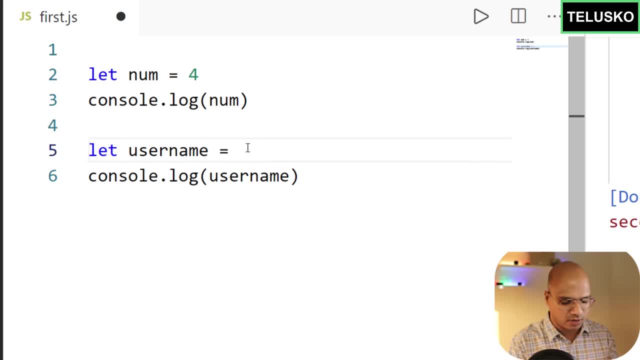 will say so. let's say, i will not put any single quote or double quote as of now. let's just write, right, right, i will say navin's phone or navin's account. so i want this to be treated as a text or a string, right? so what do you think? what should i do? should i use single? 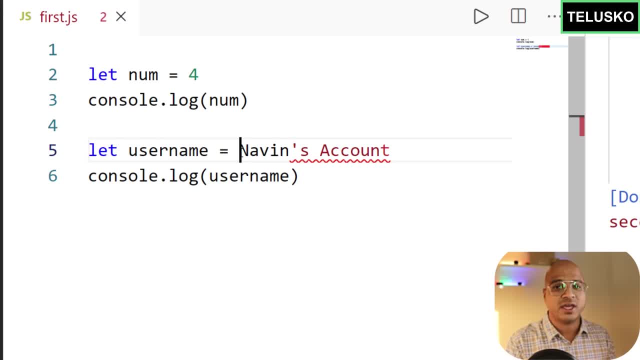 quote or double quote here. see, the problem is, if i use single quote, we already have single quote inside a text, okay. so if i put single quote, there will be a confusion. this single quote means opening a string. this single quote was supposed to be printed as it is navin's. 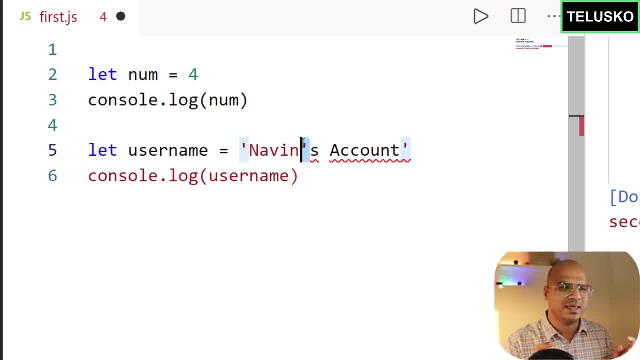 phone right or navin's account. i don't want this to be treated as the string context or string thing. so what we can do is, in this case we can use double quotes, because i just want to avoid that confusion. so we can use double quote. when do you single quote? now, let's say you have double quote. 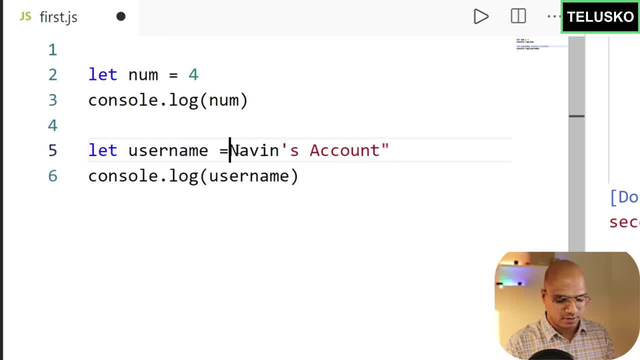 inside your text, we will be using single quote or, in general, whenever you get a chance, use single quote. it makes much more sense. okay, and there's one more thing. if you work with different languages- example c, c plus plus java- they have double quotes. so if you have, if you know, multiple 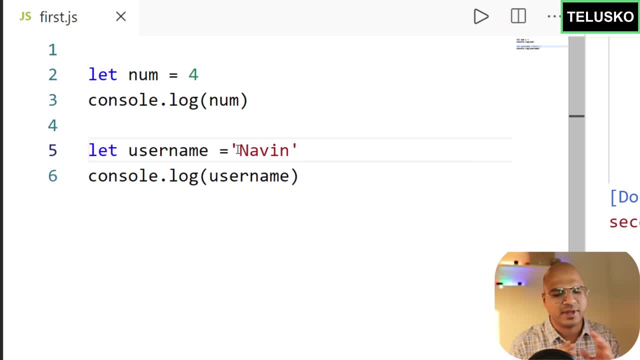 languages, you might have a tendency to write double quotes, and that's. that is completely fine. okay, so now we know how to work with two different types. we we have used numbers, we have used a string. now, likewise, we have multiple type of data. of course, we'll. 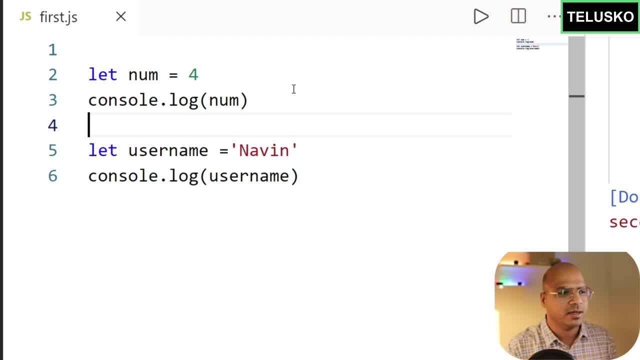 talk about that in the next video- or different type of data, but we can create any variable and we can assign any type of values there. now, why they are called as variables is because we can change the value right. so when you talk about variables, what's something you can? 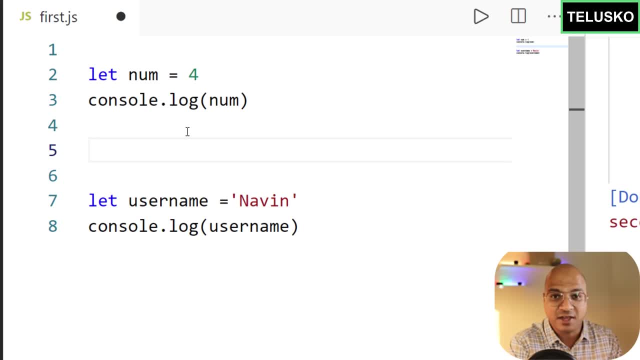 imagine, variable means it can change. in the same way, if you have a num here, we can change the value of it. so let's say i don't want num to be four anymore, i want it to be nine. do that. so let's say i will print console. so let me print num and let's see what the output is. so 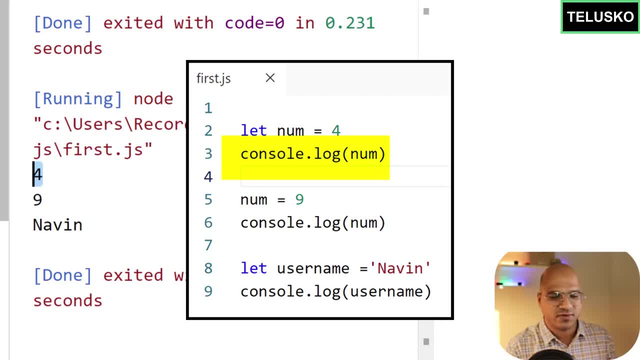 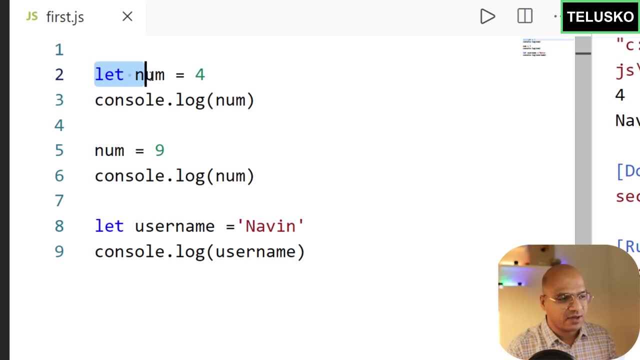 if you run this code, uh, you can see we got four because of the first line of the first console, then we got nine because of this string or this, this thing, and then we got num because of the last code here. but the question arise why we are not using let second time. it's because this time, when 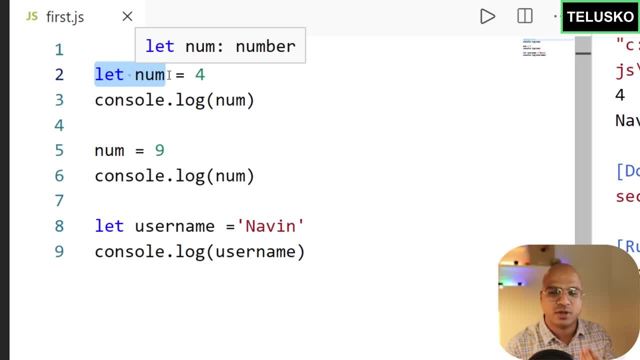 you use num for the first time, you are defining or you're declaring num. you're declaring a variable second time. you're just using it, so you don't have to declare variable multiple times. if you do that it will give you some bad words. so i will say: let num equal to nine, and if you run this code, 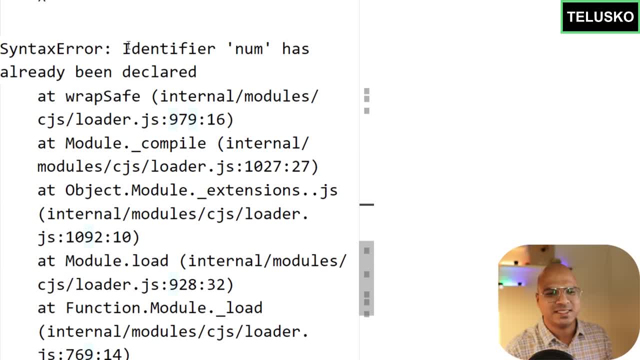 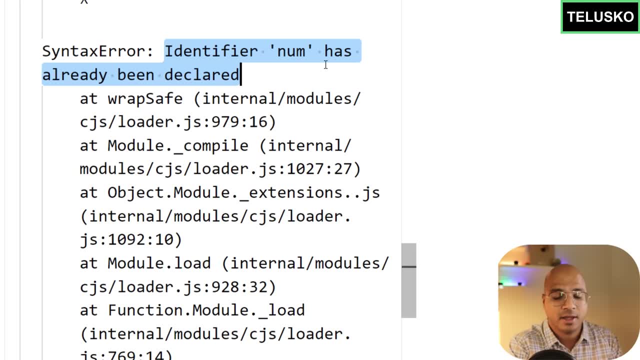 okay, and that's bad words, so you can see. you can see. it says identifier num has already been declared, and this is very important. okay, if you're starting your programming journey, you will be facing a lot of errors, as i mentioned before. that should be a part of your life. write a code, get. 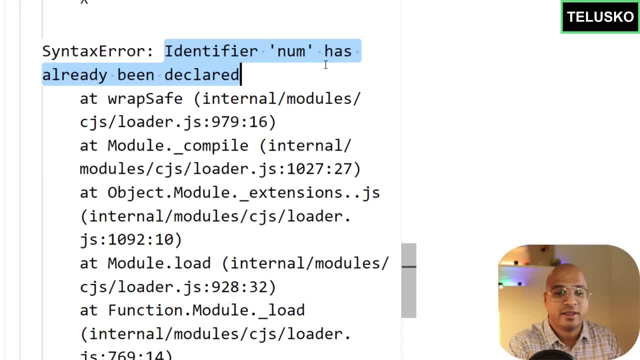 errors, solve them, which is very important, and the first step to solve a error is to read the error properly. i have seen people, okay. so, in fact, when i started coding, i used to write a code, i used to get errors, and the moment you get errors, directly jump to the code. see what, what is happening, don't jump. 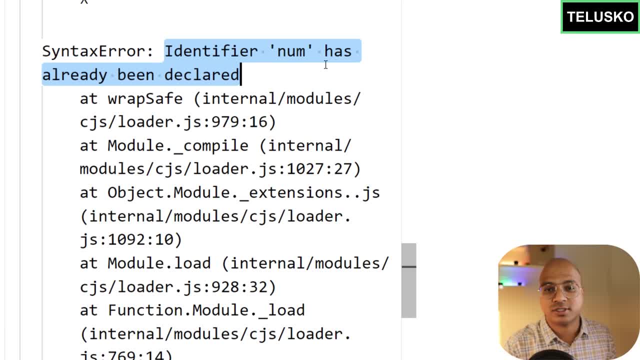 towards code, jump to the error message and see what is what's going wrong. so when you read the error, it will. it will specifically mention: identifier num has already been declared, okay, so that means you have you're declaring multiple times. so you have, you're declaring multiple times and that's what we're doing here. very important now. 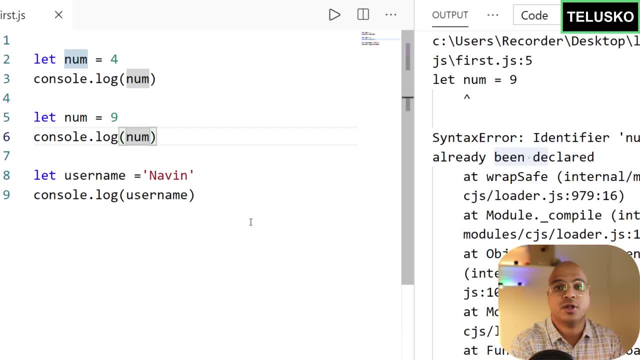 let's talk about how can you name your variable. as i mentioned before, your name should be logical. okay, don't use a, b and c- i might be using it somewhere because i'm just teaching you- but then, when you write up code for a project or for assignment, never use a variable name, which is 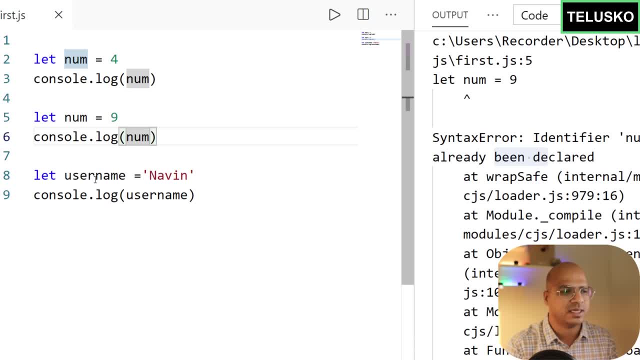 not defining itself. example: when i say num, it means something. when i say username, it means something. okay, but then are there any rules? example: i can still use a right, but are there rules that this is how your variable name should be? let's say, this is username. what if i put a dot here? not 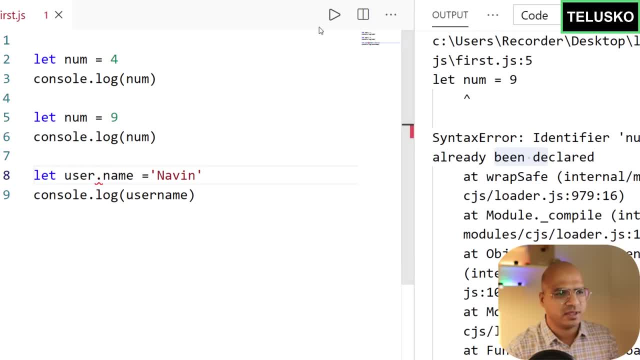 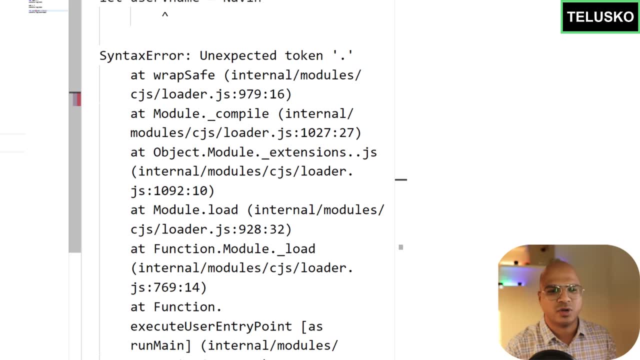 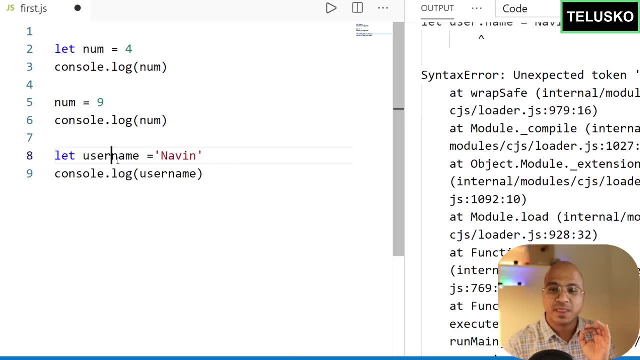 allowed. you can see we got an error there, in fact not just here. if i run this code, it will give you error data says: unexpected token. so dot is not allowed here. it has a special meaning which we'll talk about that later. so dot is not allowed. what about round bracket? not allowed. so what is allowed? 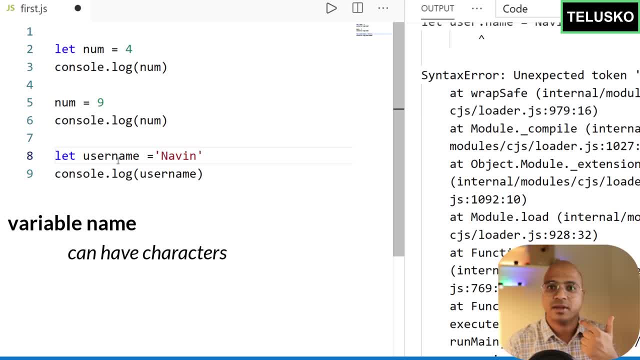 a variable name can have characters, which is there numbers as well. example, i will say username one. we can do that. okay, numbers are allowed, and you can put numbers anywhere. not the first value, the first letter should not be a number. okay, that will not work, in fact, you. 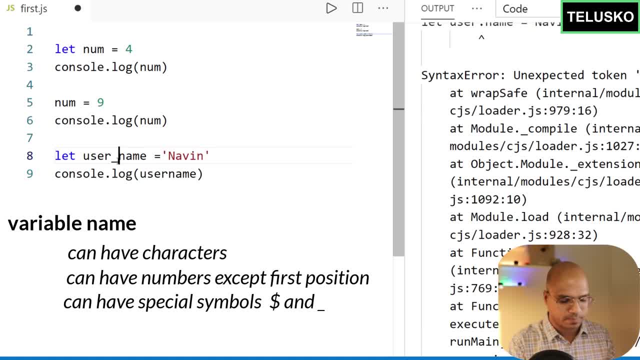 can also use some special symbol. one of them is underscore. okay, this, this is something you can do, and there's one more: you can also use dollar symbol. so you can use dollar symbol and underscore. those are the only special symbols allowed. other than that, you cannot use any other special symbol. 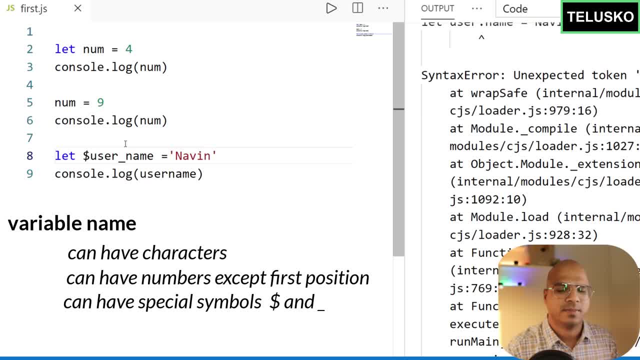 for the variable. name and numbers are allowed, but not as a first character. there's certain standards you can follow to name your variable. so whenever you have variable which has two words- example, if you look at this username here you can see there are two words right- user and name- and what happens? 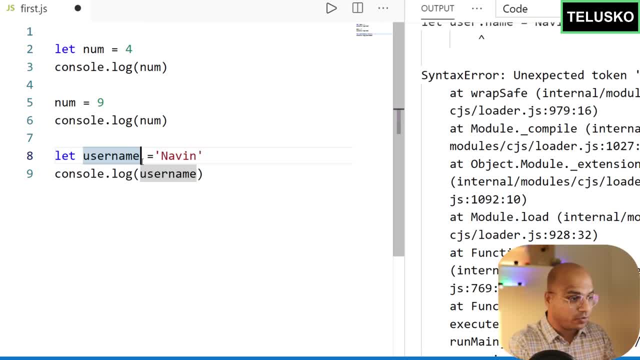 is the moment you start reading something. when you, when you read a code, it should be readable right now. if you have these two words, there are two ways you can differentiate between these two words: words, because in English we use spaces right and spaces are not allowed here. so